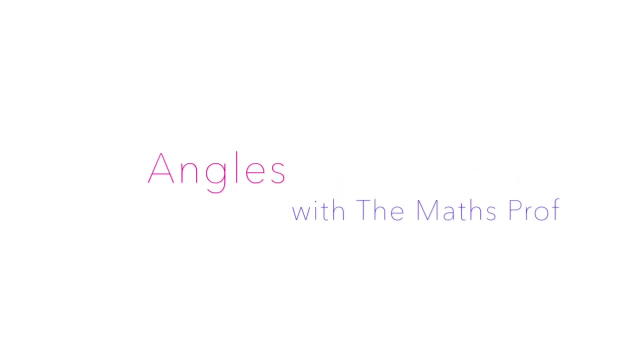 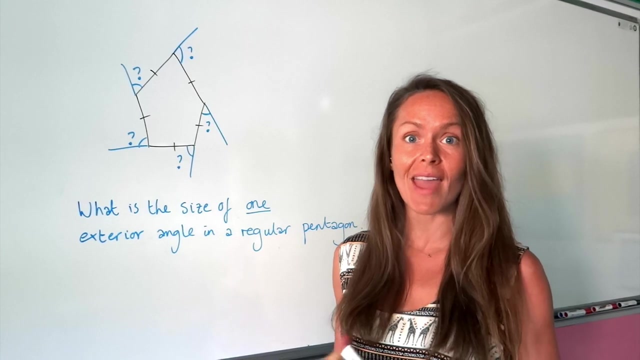 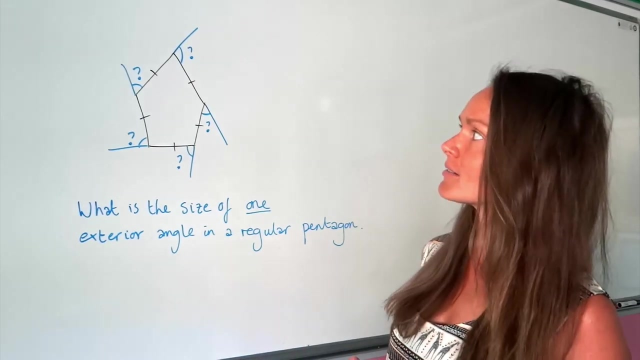 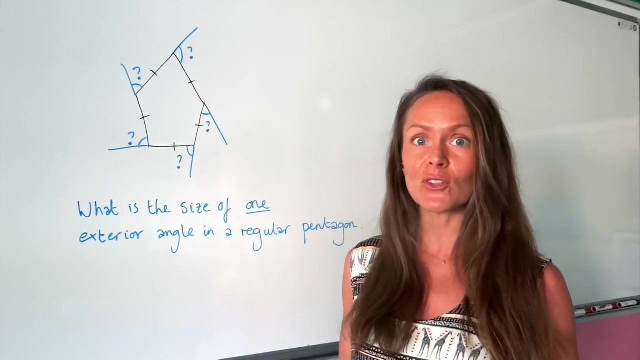 Hey guys, in this video I'm going to talk to you about exterior angles in polygons. So remember, polygon is just a fancy word for shape and exterior angles. well, they're these angles here, outside of the shape. Okay, Something really important you need to remember. 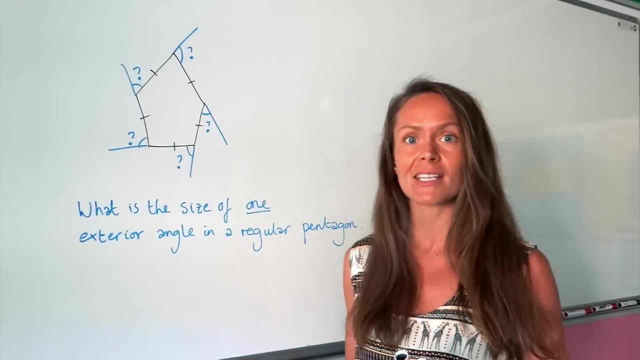 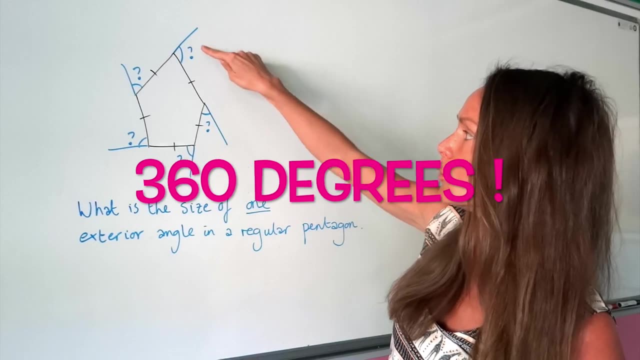 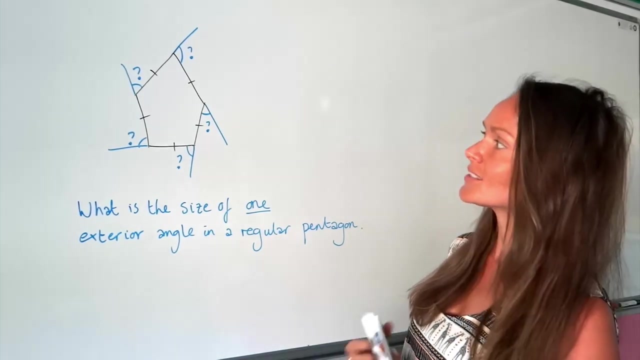 before you can have a go at these questions is: all of the exterior angles, in absolutely any shape, always add up to 360 degrees. Okay, So all of these outside angles will always add up to 360 degrees, no matter what the shape. So in this question we've got a regular 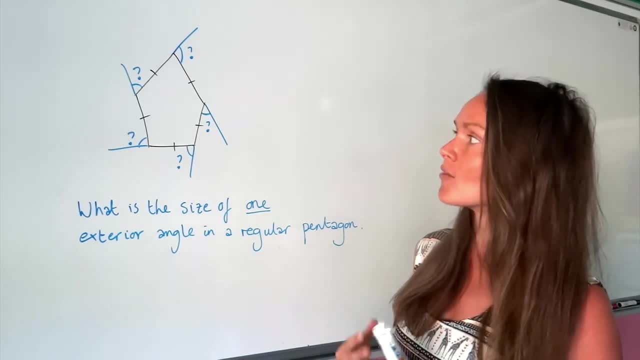 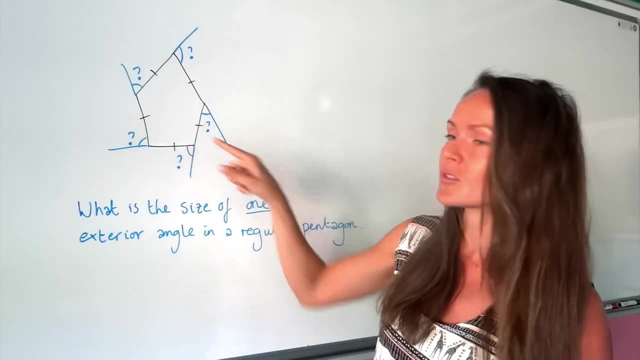 pentagon. So a pentagon is just a five-sided shape, and regular just means that all of these lengths are the same and it also means all of the angles are the same. So all of the angles are the same inside the shape, which also means all of the exterior angles. 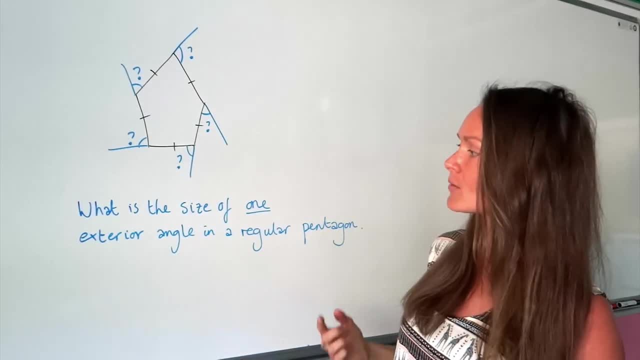 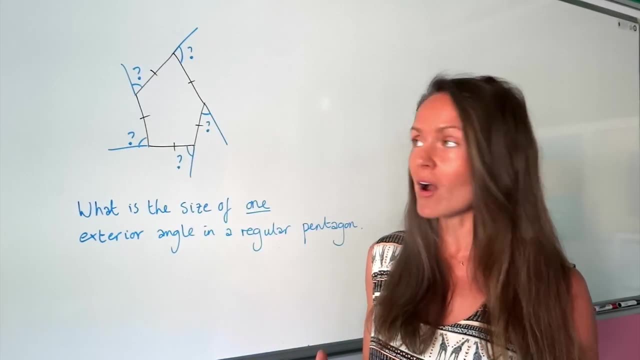 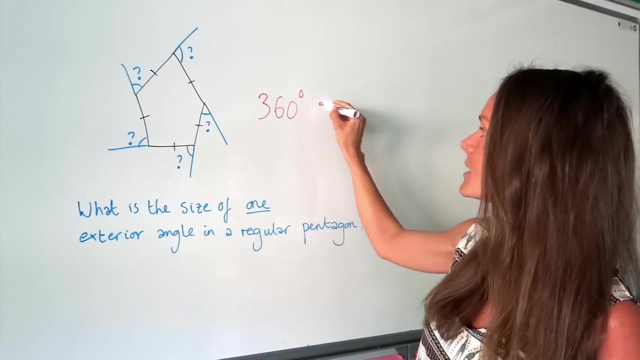 are equal in size too. So if we have to work out the size of just one of these exterior angles, so one of these here, what you need to do is divide 360 degrees, because, remember, that's the total, that's what they add up to. We have to divide by the number that there 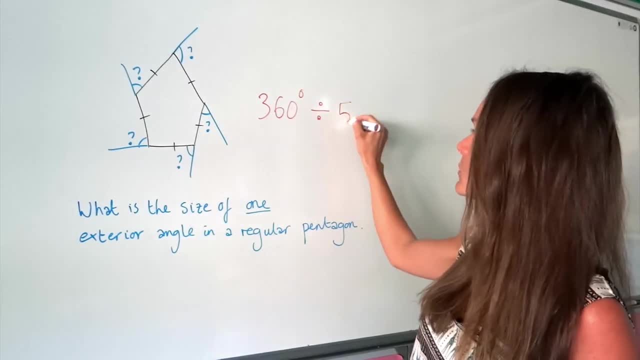 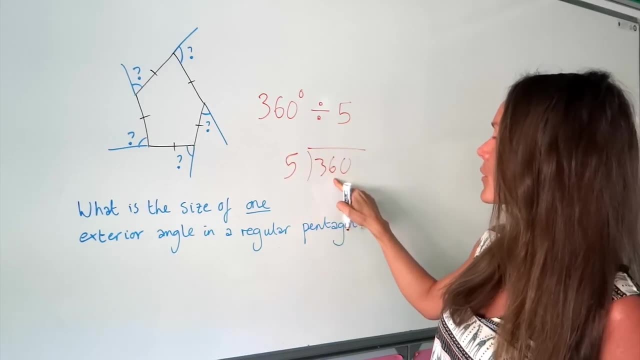 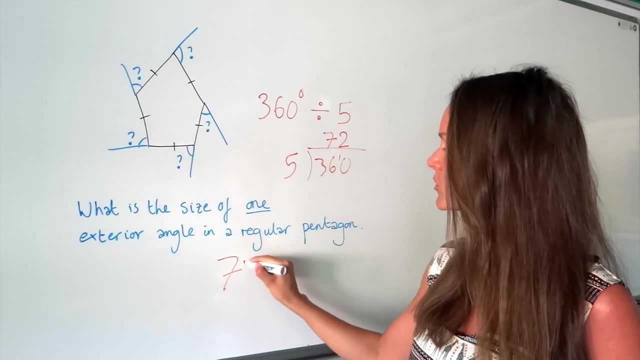 are, and there are five all together. So we have to divide 360 by the number that there are by five. So if you work that out, fives into 36, well, that's seven, and there's one remainder, fives into 10, two. So that's the answer to the first question. It's 72 degrees. 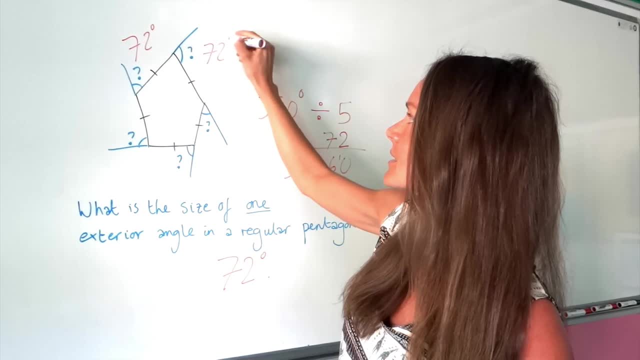 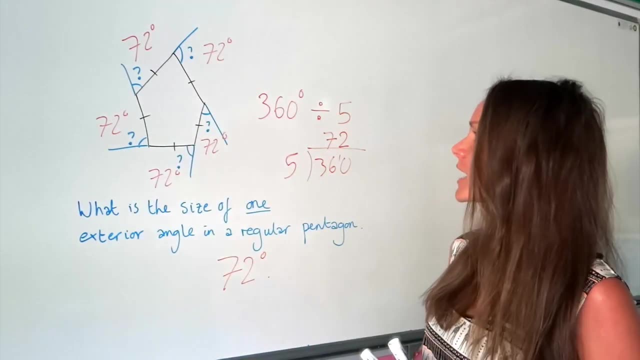 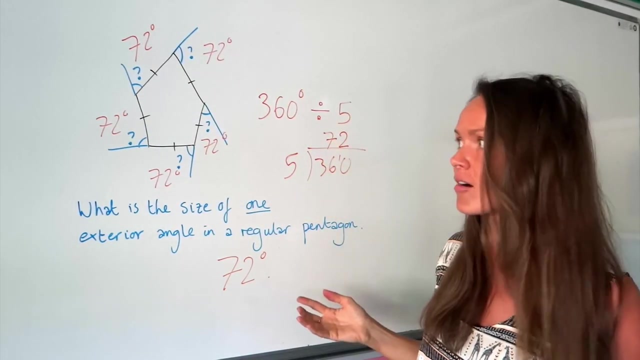 So each of these exterior angles is 72,. okay, Because, remember, they're all the same, because it's a regular pentagon. Okay, so it's just always 360 degrees, because that's the total divided by However many there are, And that will work for any regular polygon, any regular shape. 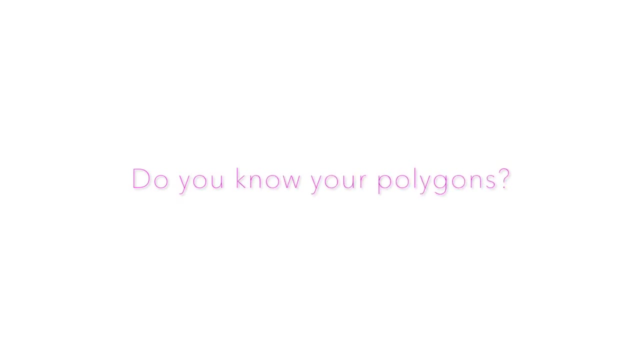 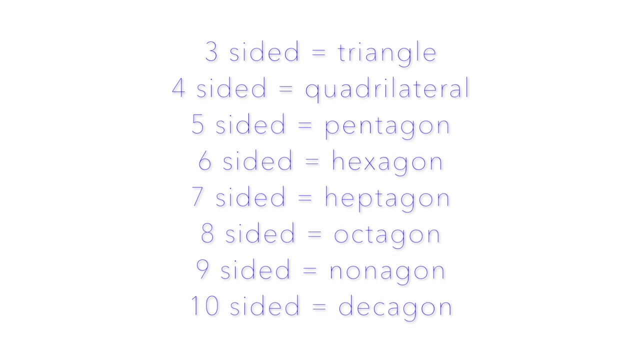 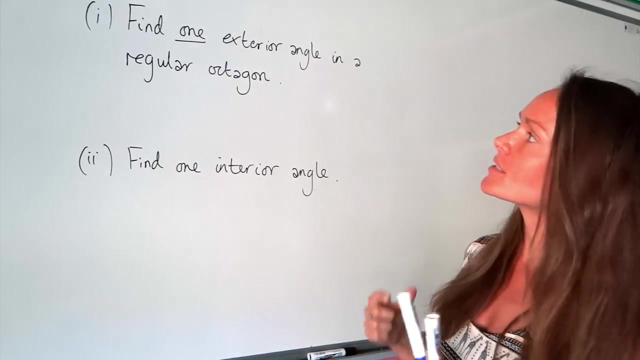 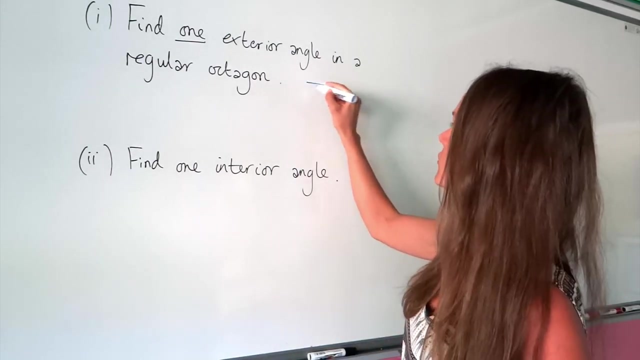 Okay, on to the next one. Okay, so this time there's no diagram, but that's fine. It says: find one exterior angle in a regular octagon. So an octagon is an eight-sided shape. So I'm just going to do a little sketch here just so you can see what's going on. Okay, 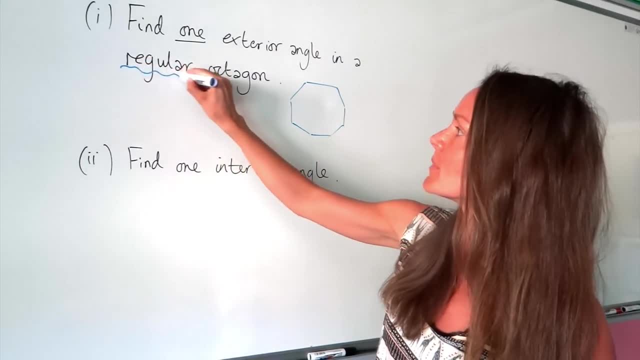 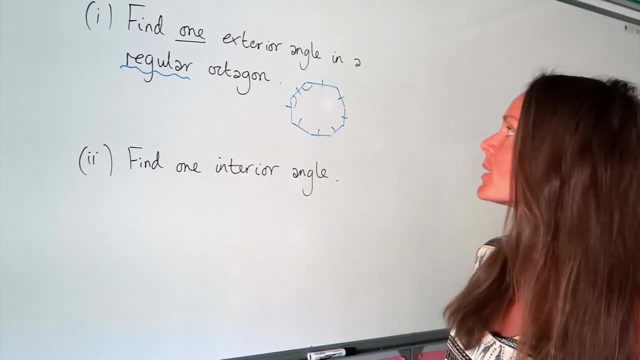 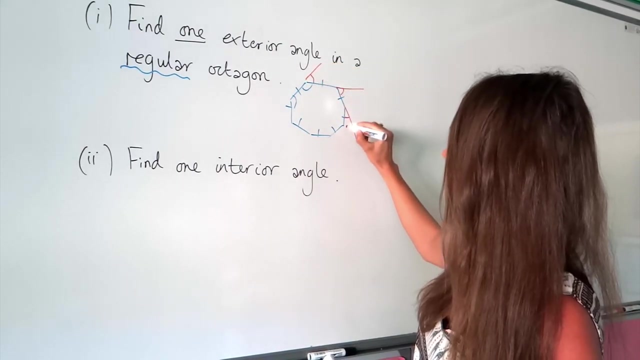 it doesn't need to be accurate And remember it's regular. So that means all of the lengths are equal in size, all of the angles are equal in size And remember all of the exterior angles, those ones outside the shape, they always add up to 360.. Okay, so if we need 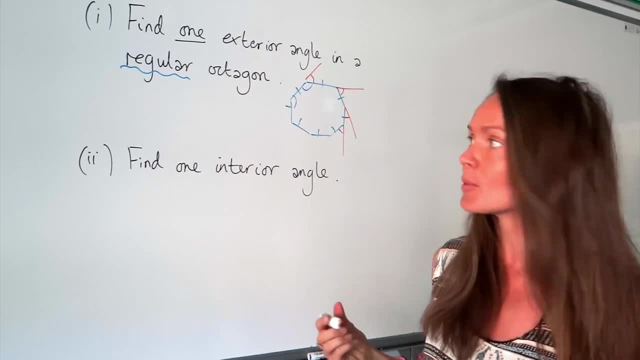 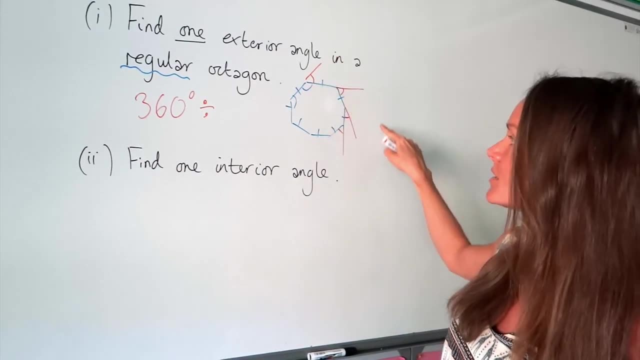 to find one of those exterior angles, just like before, we need to divide by the number of angles. So if we need to find one of those exterior angles, just like before, we need to divide 360 by however many there are, And this time because it's an octagon, which is an. 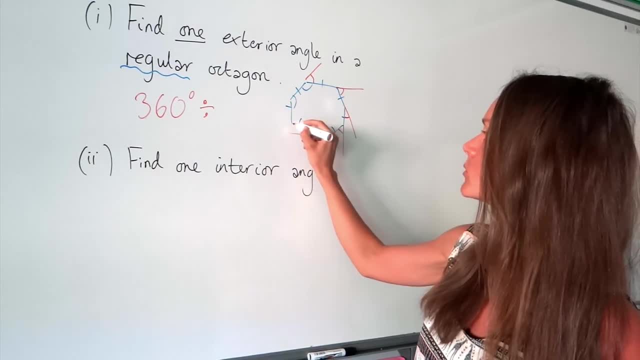 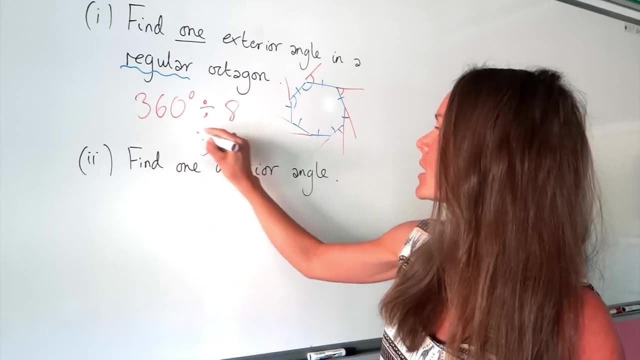 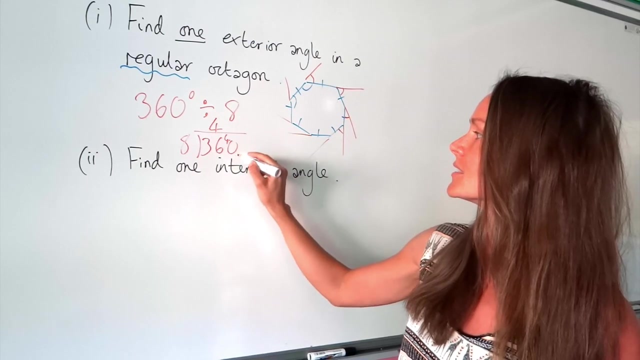 eight-sided shape, there will be eight exterior angles, So we need to divide 360 by eight. Okay, so I'm going to work this out. So eight into 36 goes four times with a remainder of four, And eight into 40 goes five. So that's the answer to the first question. One of the 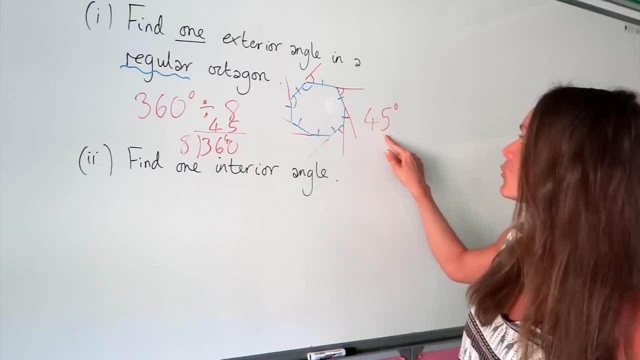 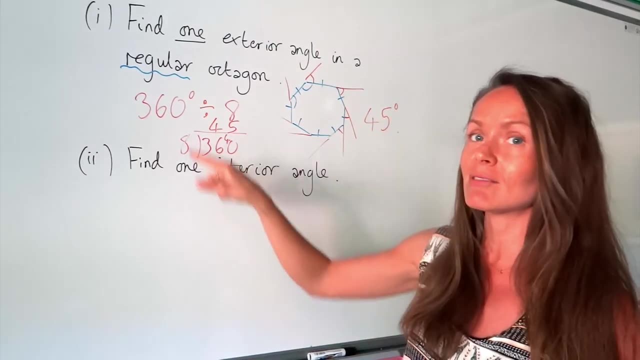 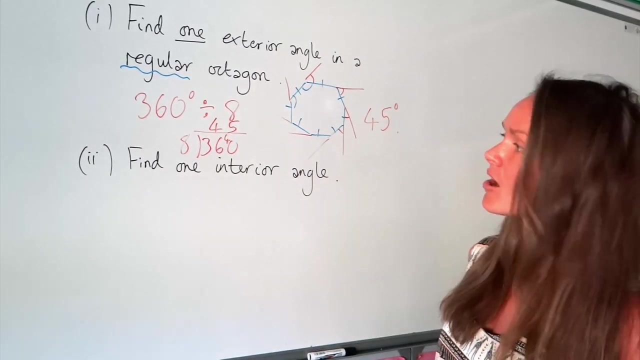 exterior angles in a regular octagon is 45 degrees. So it's exactly the same method as before. You're just dividing the total, which is always 360, divided by eight, because there are eight exterior angles altogether. So next it asks us to find one interior angle. 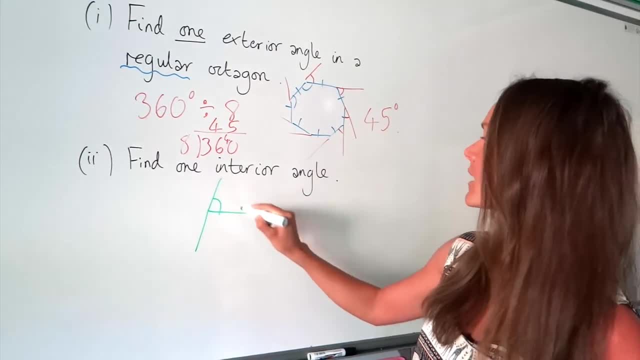 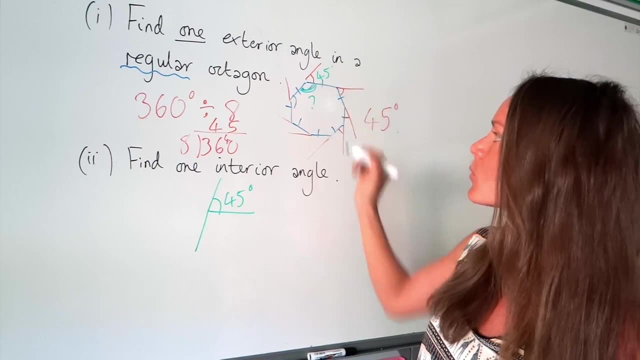 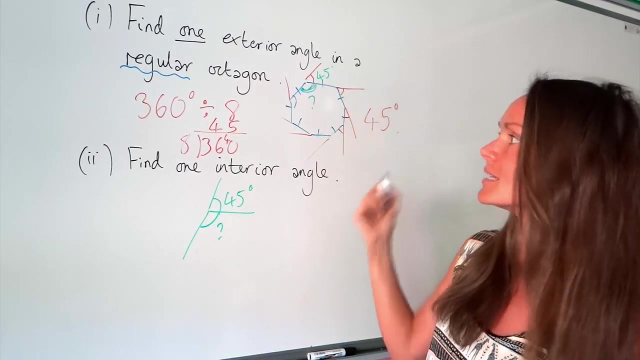 So we just worked out that the exterior angle was 45 degrees. Okay, so outside the shape. Now the interior angle was 45 degrees. So we just worked out that the exterior angle angle is this one inside. So we're trying to work out this one here. Okay, So the angle inside the 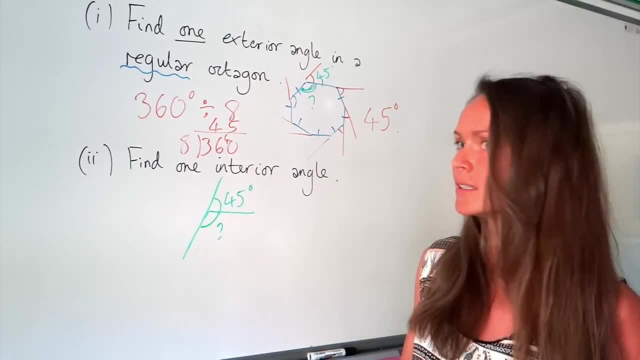 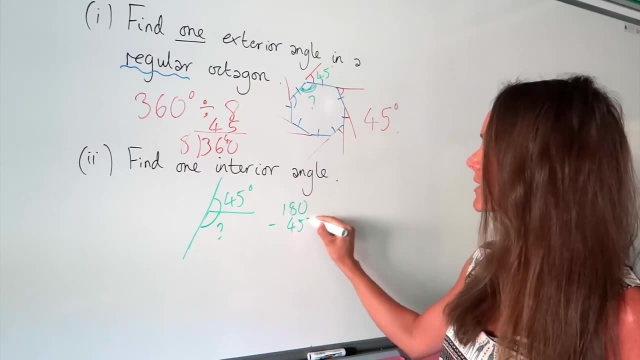 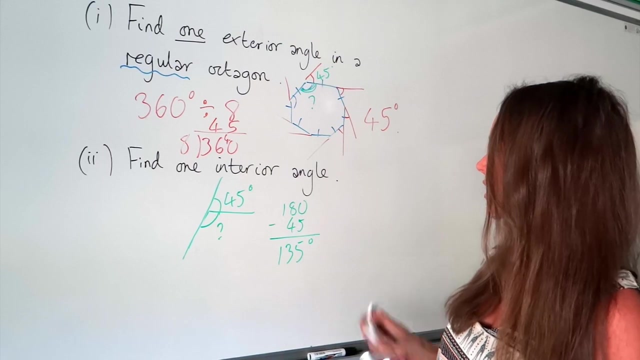 regular octagon. Well, because this is a straight line, angles on a straight line. they always add up to 180 degrees. So you just have to subtract your exterior angle from 180, which gives 135 degrees. So that's the answer there. So you just need to remember that an interior and an exterior.